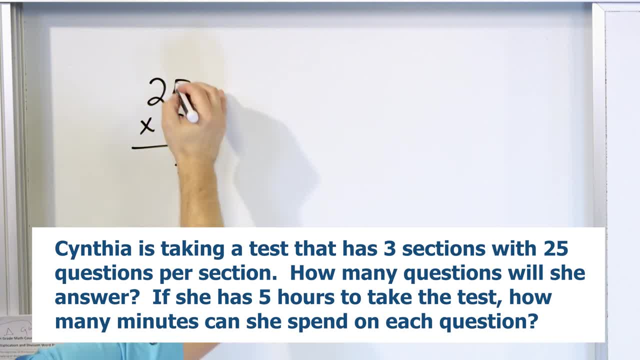 three, because that's three sections, And then three times five is 15.. And then two times three is six. One more is 75 questions. So during the test she will answer a total of 75 questions. Now the next thing says: if she has five hours to take the test, how many minutes can she spend? 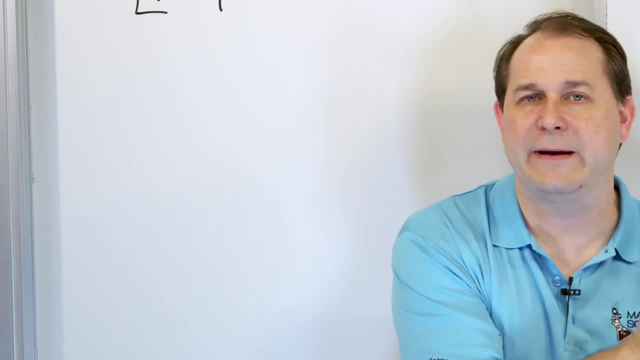 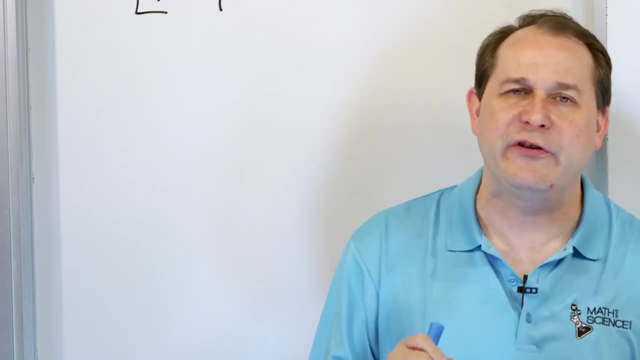 on each question. Notice it tells you there's five hours that she's spending on the test, but they don't ask you how many Hours per question. They ask you how many minutes per question. So the first thing we have to do is: 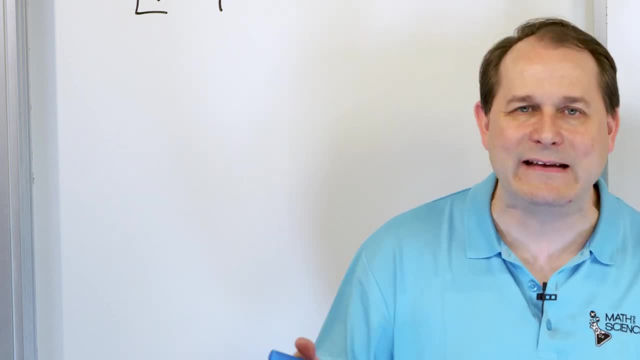 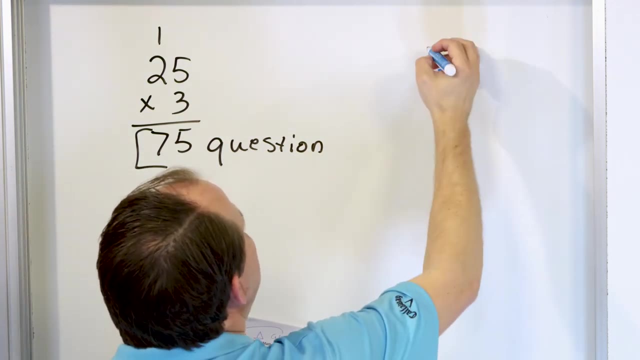 figure out if we have five hours of time, how many minutes is that? So we have five minutes of time, but we know that there's 60 hours and 60 minutes in every hour. So 60 times five, that's how many. 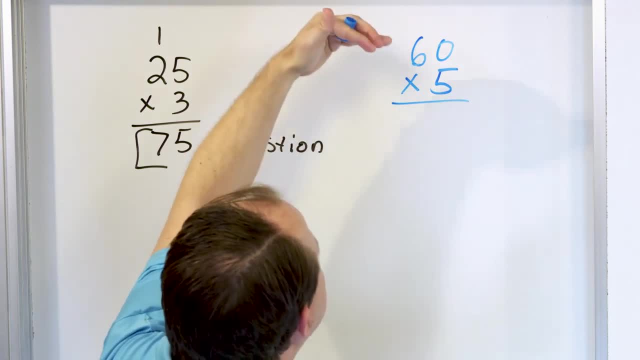 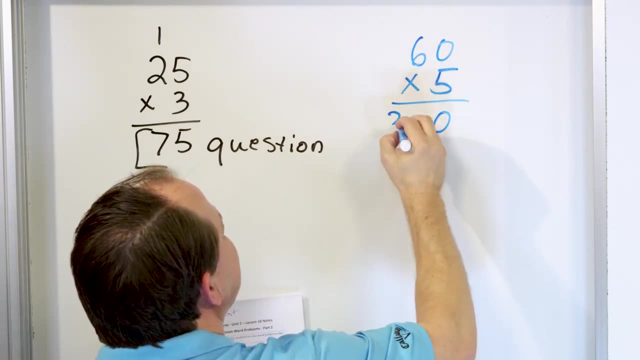 minutes. we're going to have 60 minutes in the first hour, 60 minutes in the second hour, 60 minutes in the third hour, in the fourth hour, in the fifth hour. So we multiply five times zero, zero and six times five is 300. 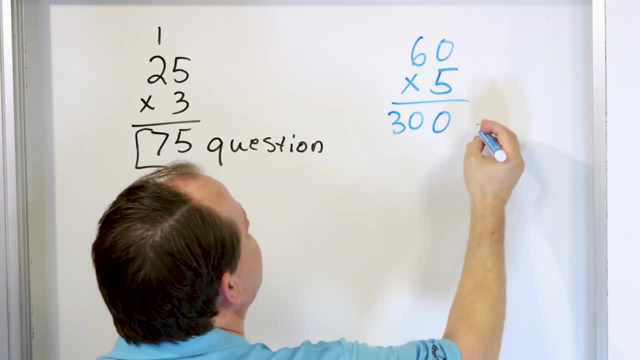 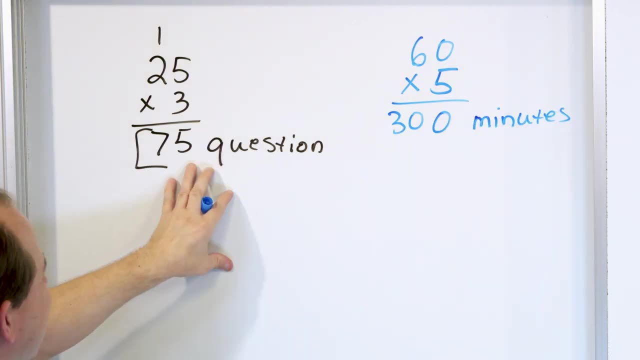 So we have 300 seconds, So we have 300 minutes total to take the test. So if we have a total of 75 questions and we have a total of 300 minutes, how do we figure out how many minutes we can spend on this thing? What we're really trying to figure out is how many minutes per question, Because 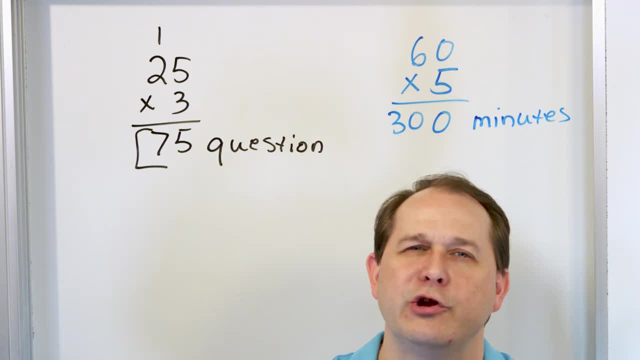 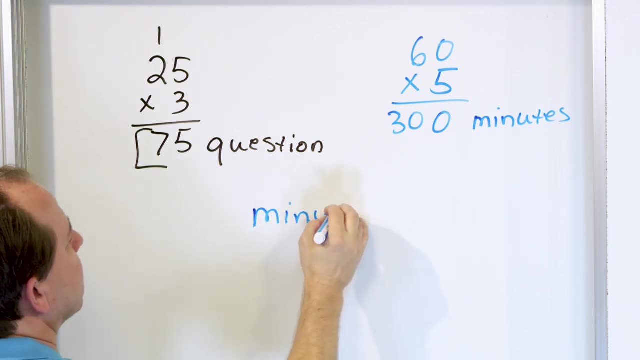 really when it says how many minutes can she spend on each question. another way to phrase that would be how many minutes per question. We want a unit of minutes per the line means per question. All right. So how many minutes do I have? I have 300 of them. How many questions do I have? I have 75 of them. You see, I've kind of 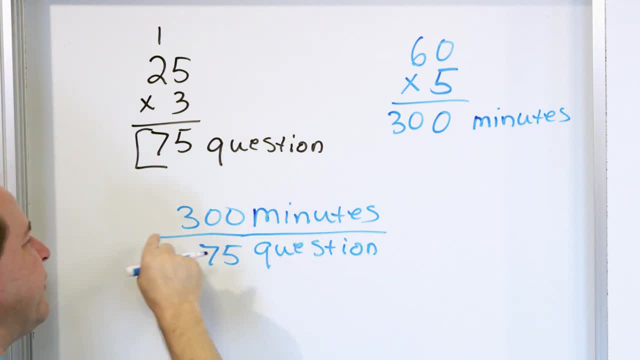 made a little unit here. So 300 minutes, 75 questions. If I divide these numbers, I will get a unit of minutes per question. That's exactly what the thing is asking me to do. So 300 divided by 75.. 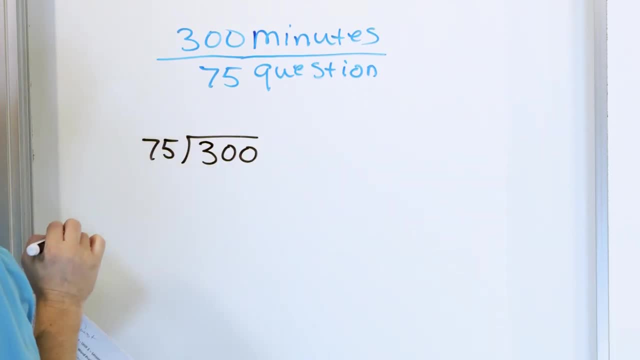 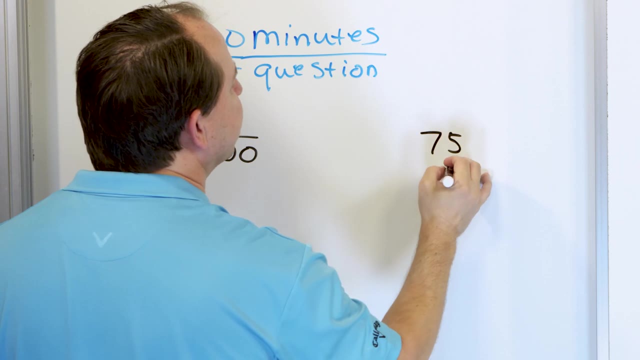 All right, How many am I going to fit here? I'm not sure if it's times one or times two, or times three or times four. Let's just try 75 times four. Five times four is what- 20.. And then seven times. 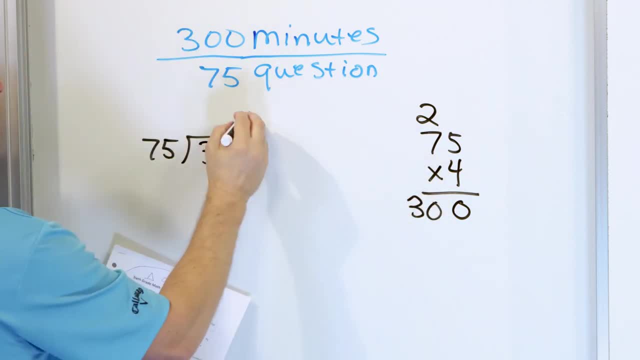 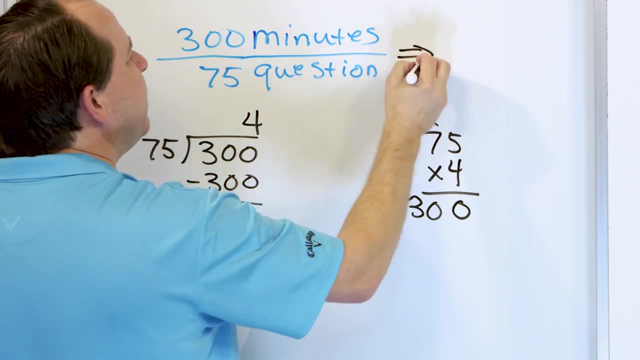 four is 28,, 29,, 30. It's exactly equal to 300.. So four- we just said it's equal to 300.. Remainder zero, We get an answer of four. So what this means is when we do this division, we get an answer of. 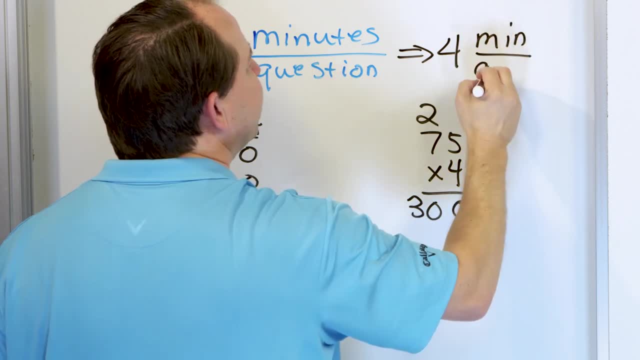 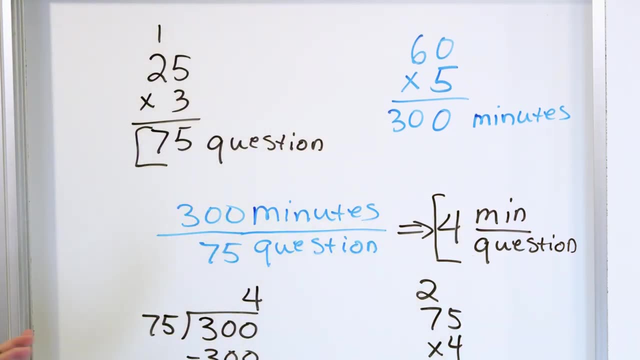 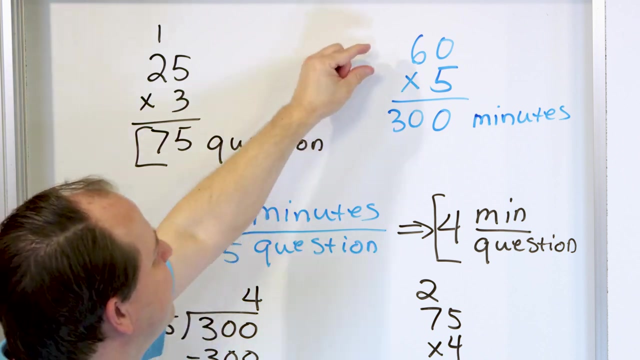 four minutes Per question, which is what we want to calculate: How many minutes per question. So we answered both questions. She's going to answer 75 questions and she's going to spend four minutes on each question. The real thing that you had to think about is you have to take the number of hours. 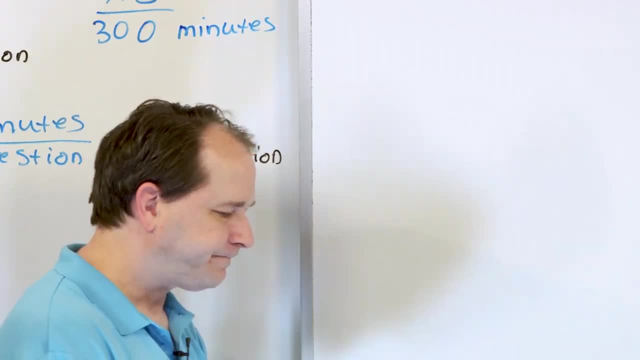 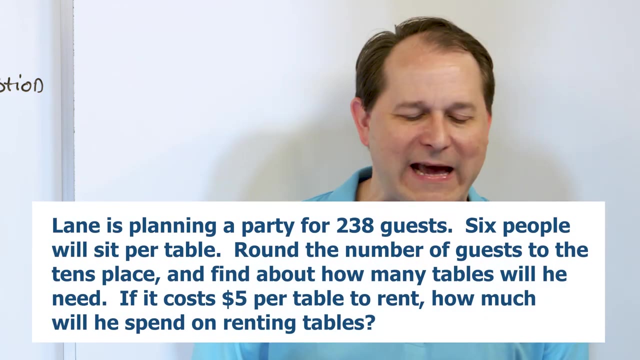 given and convert it to minutes by multiplying by 60.. All right, Let's take a look at problem two. It says Lane is planning a party that will have 238 guests. He wants to sit six people to a table at the party By rounding the number of people at the party to the tens place. 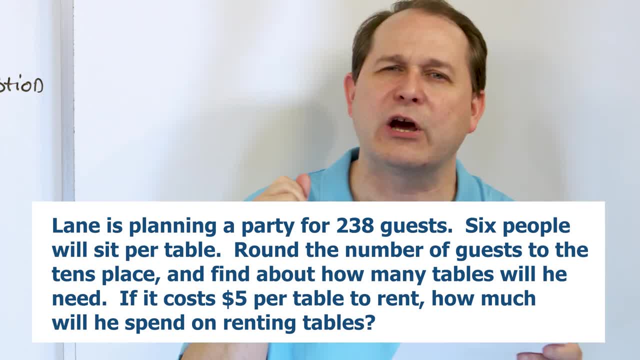 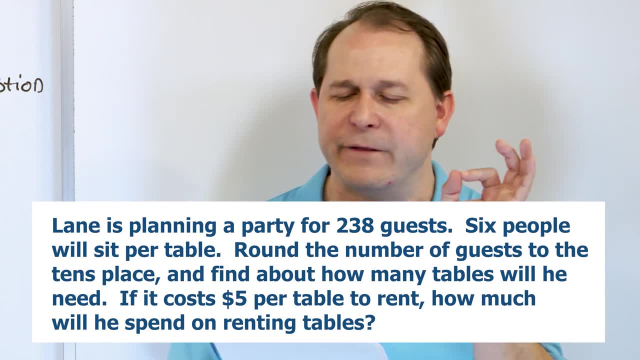 find out about how many tables will he need. If it costs $5 to rent every table, about how much will he spend on renting tables? So again, there's two questions here. The first one is, by rounding the number of people at the party to the nearest tens place, find out about how many tables he 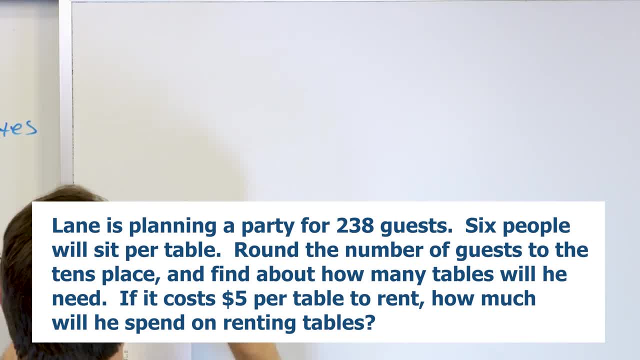 needs. All right, Well, first of all, it tells us to round the guests right, So we have 238 guests. We want to round to the nearest tens place. This is the tens place, So we can go up to 240, or we can. 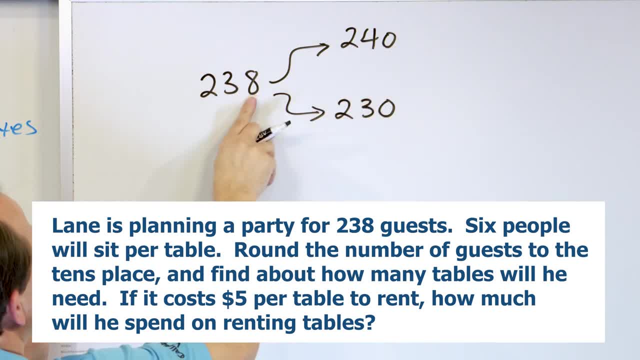 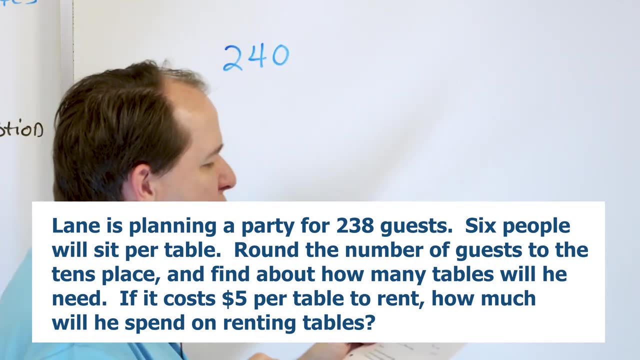 round down to 230.. How do we decide? This number next door is larger than or equal to five, So actually we're going to round up to 240.. All right, So now we know we have 240 guests. This is a rounded estimate, right? And we know we want to do six people to a table, So we're going to 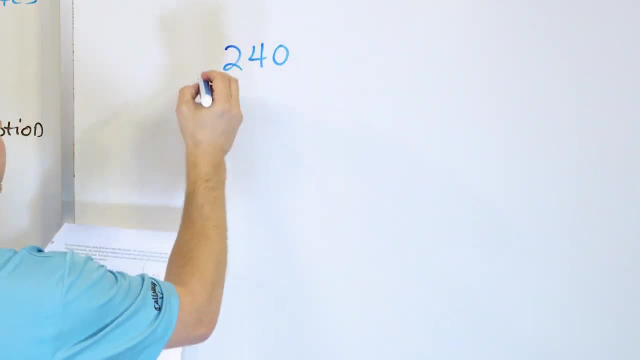 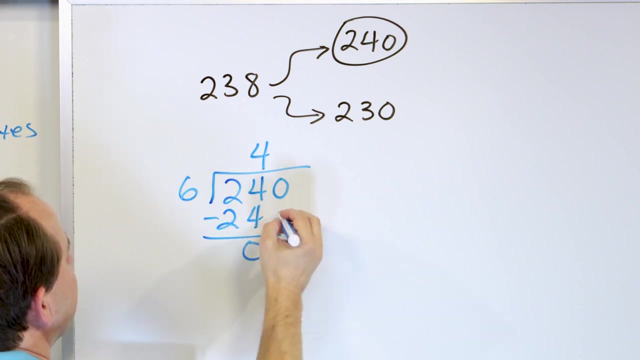 divide by six. How many groupings of six can we make when we start with this? So we divide by six, Six times what is 24? Six times four is 24.. Subtract, get a zero. drop this down, And now we. 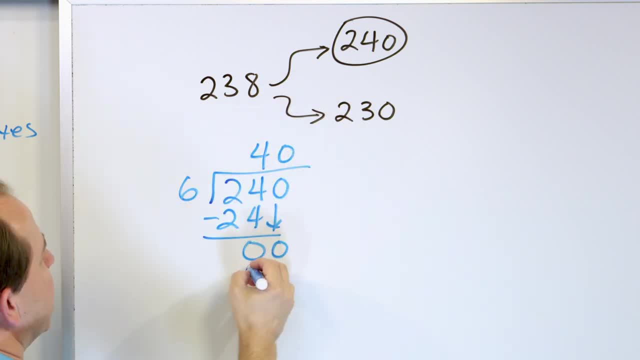 have six times what is zero. The only thing that works is zero. Multiply, get a zero, subtract and finally get a zero, All right. So the answer to this question is: when I start with a rounded estimate of guests of 240 guests and six people per table, then what I'm going to have. 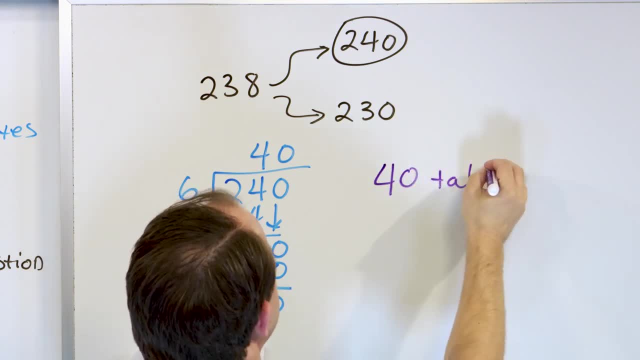 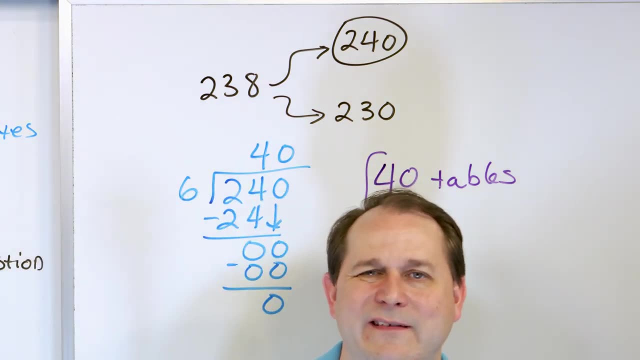 I'm going to need 40 tables because I have 40 groupings of six. I'm going to need 40, 20 tables here. Now the next question says: if it costs $5 to rent every one of these tables, how much money am I going to spend? Well, I'm going to have to take the 40. 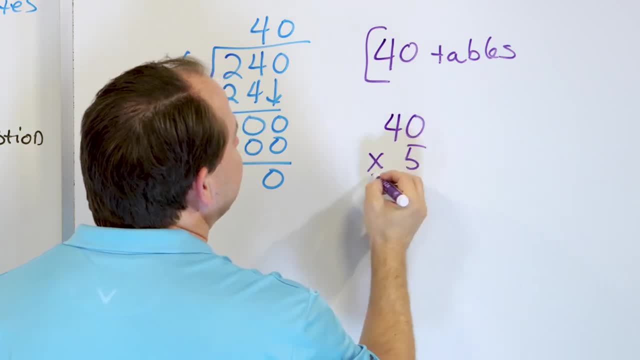 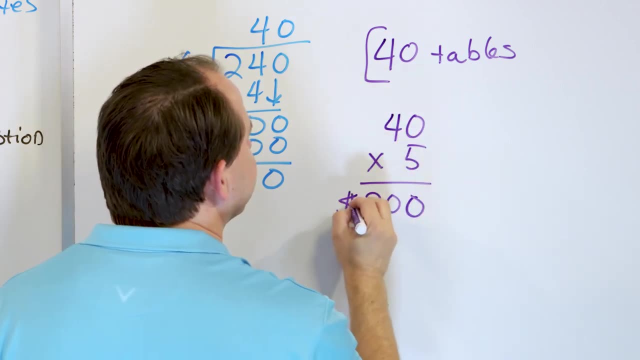 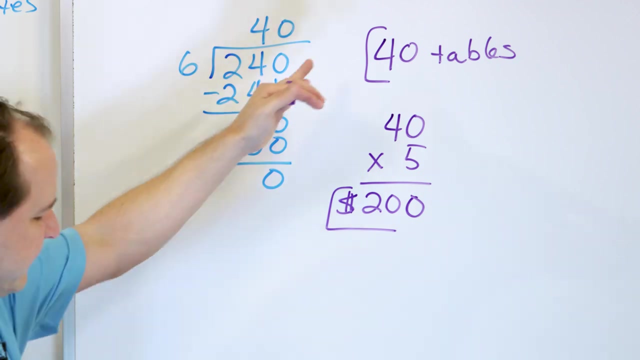 tables that I know I'm going to need to rent and multiply by five, because it's $5 for every one. Five times zero is zero. Five times four is 20.. So it's $200 total, because it's 40 tables times $5. So the answer is $200 total: 40 tables. $200 is what I'm going to spend to rent them. 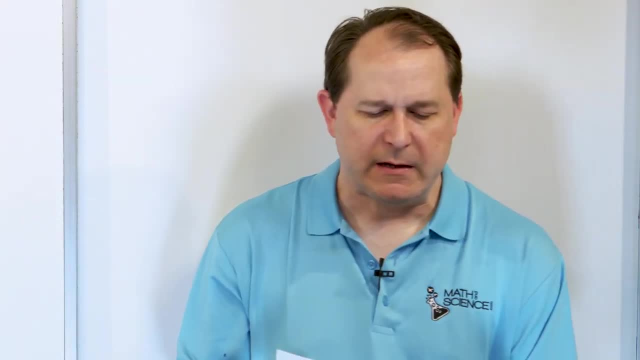 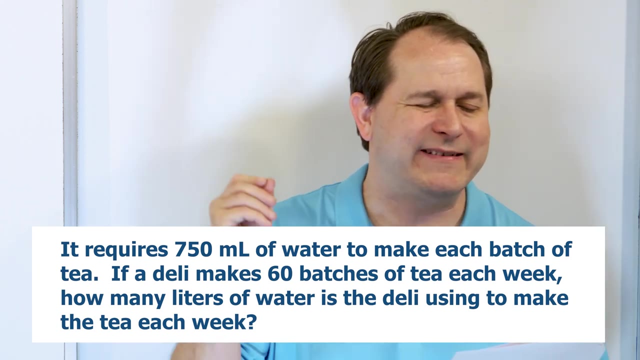 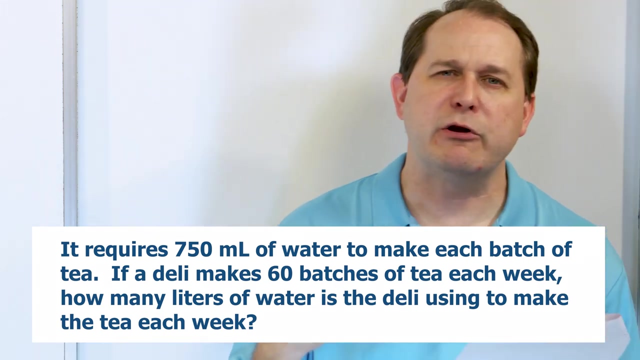 All right, Take a look at problem number three. It requires 750 milliliters of water to make a batch of tea. If the deli makes 60 batches of tea every week, how many liters of water is the bakery using to make the tea? So we want to know how many, how much water we're using. but the tricky 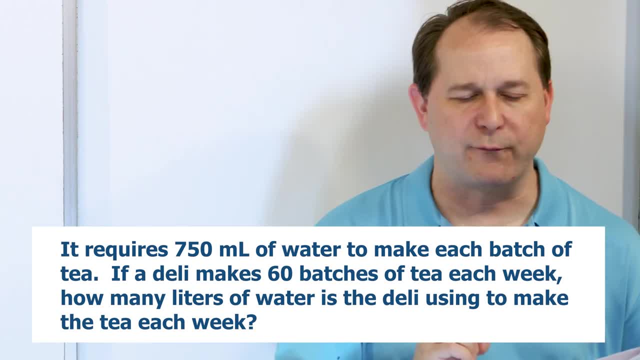 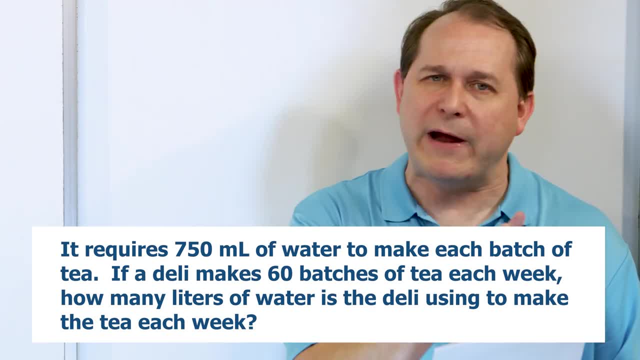 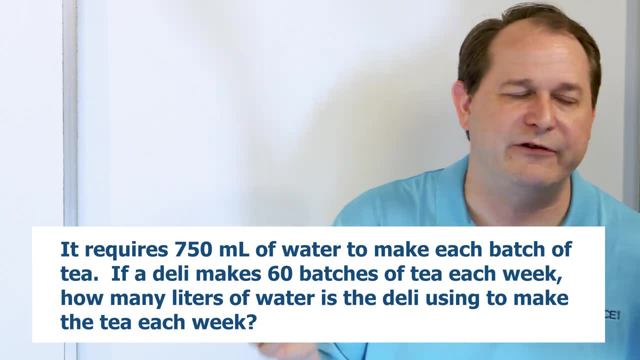 liters. That's a different unit than milliliters, So let's break the problem apart. The first thing we're going to do is take 750 milliliters and multiply by 60, because there's 60 batches. That will tell us how many total milliliters we need of water. So we'll take the 750 milliliters. 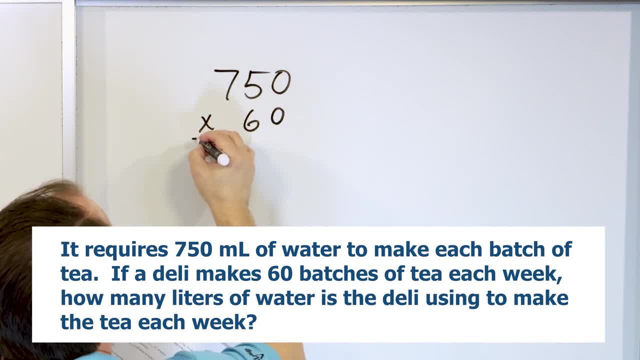 of each batch, and then we will multiply by 60 batches. This will tell us how many milliliters of water we need altogether. Now, zero times zero is zero. Zero times five is zero. Zero times seven is zero. Drop a zero. Zero times five is zero. Zero times seven is zero. Zero times seven is zero. 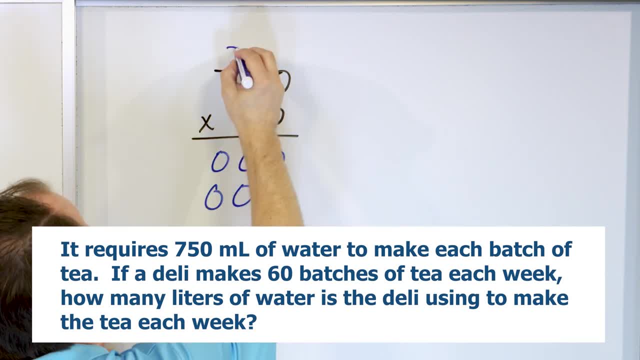 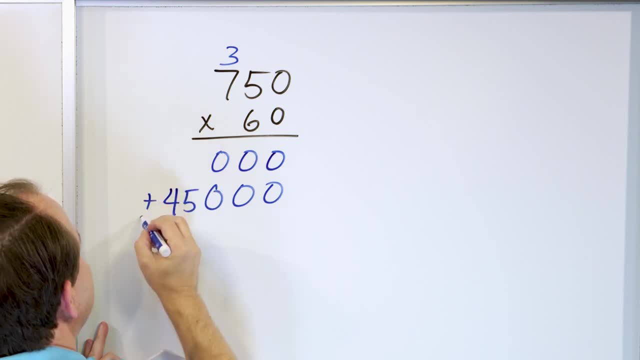 Six times zero is zero. Six times five is 30. Carry the three Six times seven: 42,, 43,, 44,, 45. There's 45. And then we add these together And of course it's just going to. 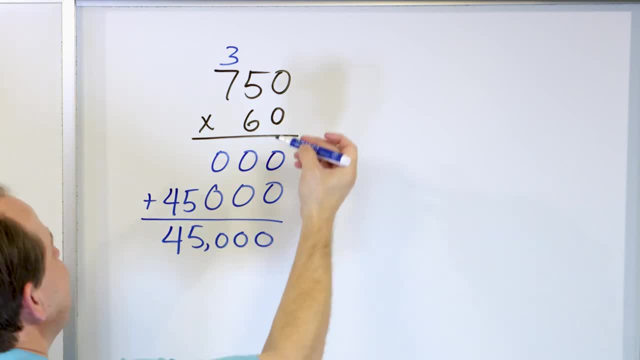 be 45,000.. And what have we calculated? 750 milliliters per batch, And then this is batches, so the total thing is milliliters. This is in milliliters, But I don't want milliliters. 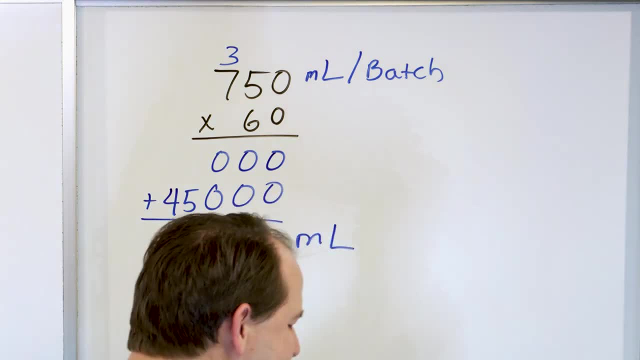 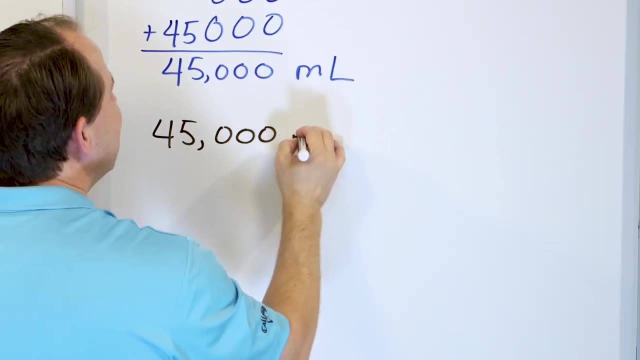 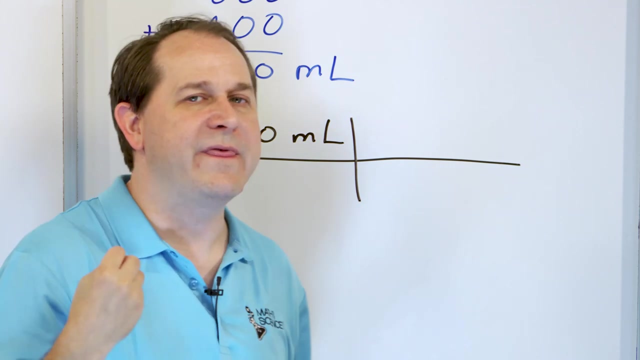 This is how many liters of water. How many liters of water? So we have to do a unit conversion. So the way you do it is you write down what you're given: 45,000 milliliters. Now we learned before how many milliliters are in a liter. There are 1,000 milliliters. 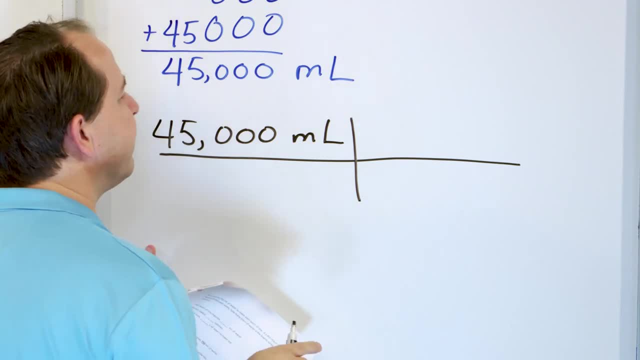 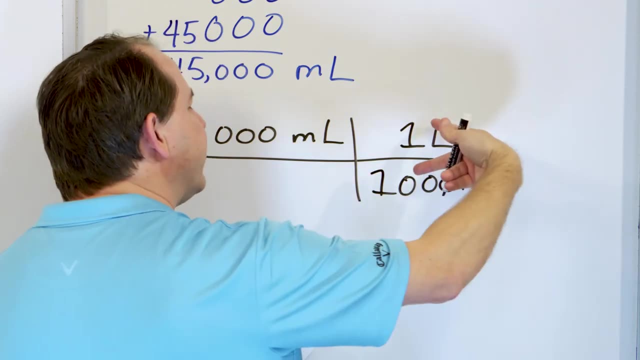 in a liter right. So we have to write a little conversion factor here. So there are 1,000 milliliters in every one liter. These go together. I don't want to flip it over because nothing will cancel if I flip it over, But if I write it like this: 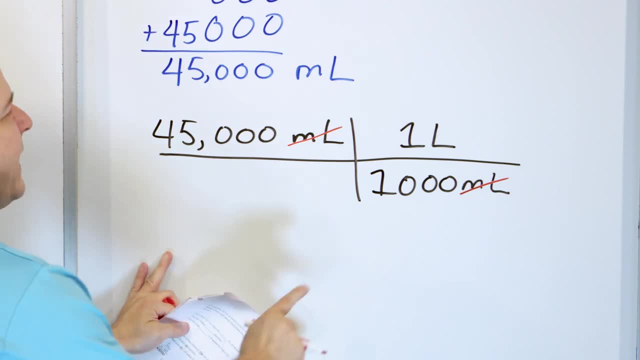 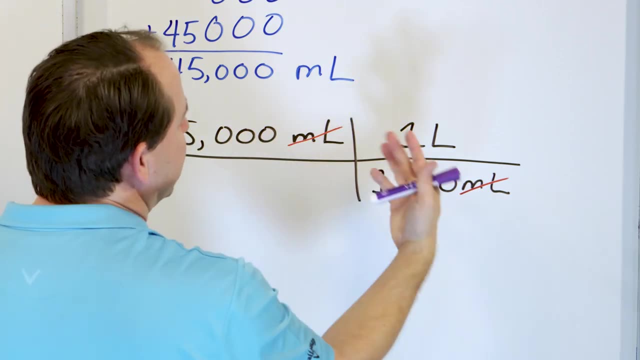 the milliliters on the top will cancel with the milliliters on the bottom, And the only thing I'll have left is liters, which is what I want. The reason I'm doing this is because it tells me to take the 45,000 times 1,, which does nothing, and divide by 1,000.. 45,000, I'm going to divide. 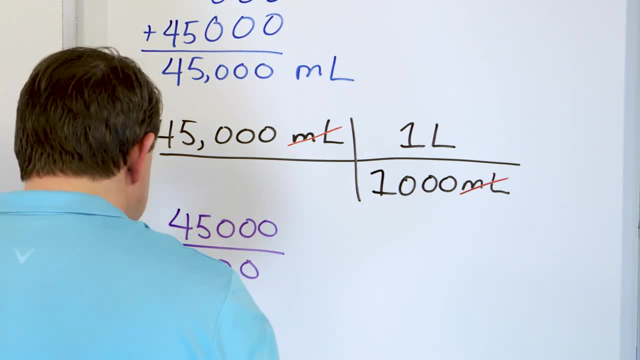 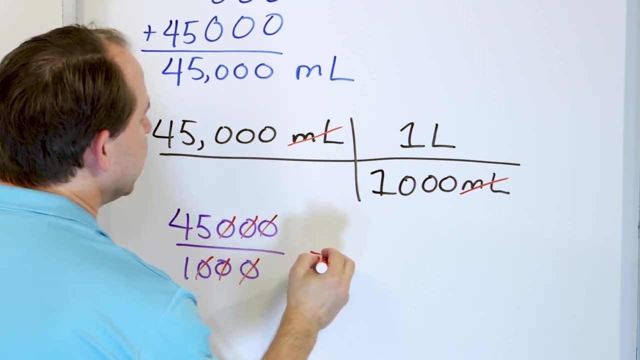 by 1,000, like this. And the reason I'm doing that is because this 0 will cancel with this one, this one will cancel with this one and this one will cancel with this one. I have 45 divided by 1,. 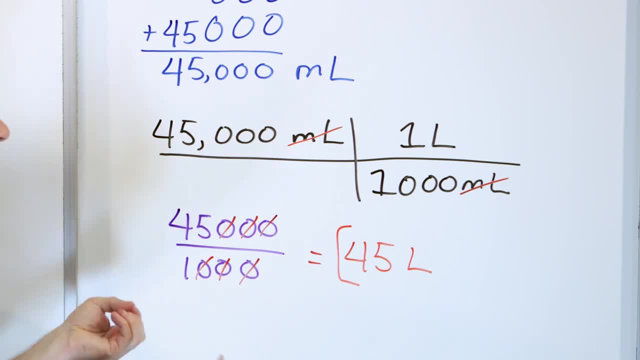 and this one will cancel with this one, and this one will cancel with this one and this one will cancel with this one. So if I have 45,000 milliliters, I will need 45 liters of water. It makes sense really. 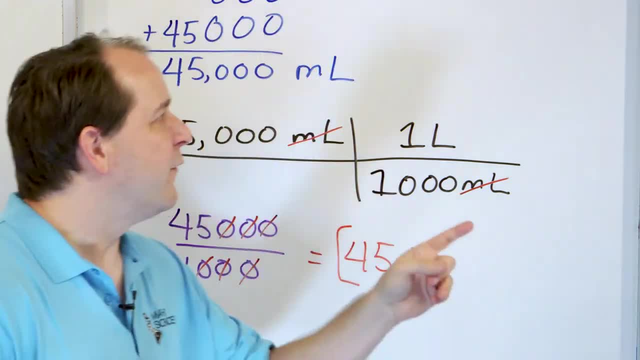 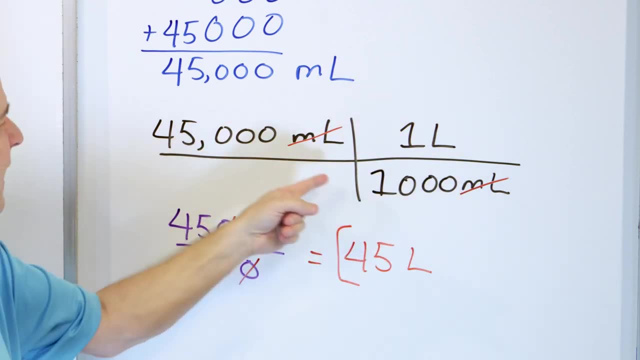 because you know, 1,000 milliliters is for 1 liter. So if I had 45,000 milliliters I must have 45 liters. This whole thing here is just telling you to divide these numbers, because it's oftentimes 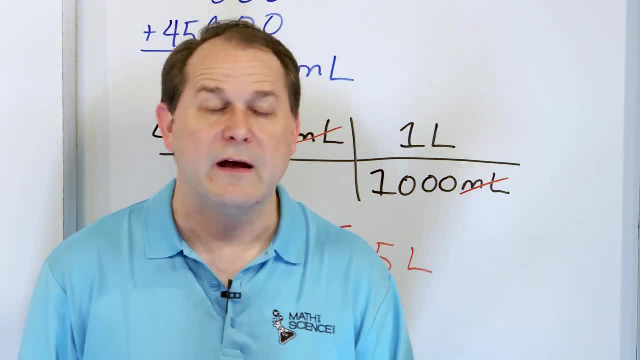 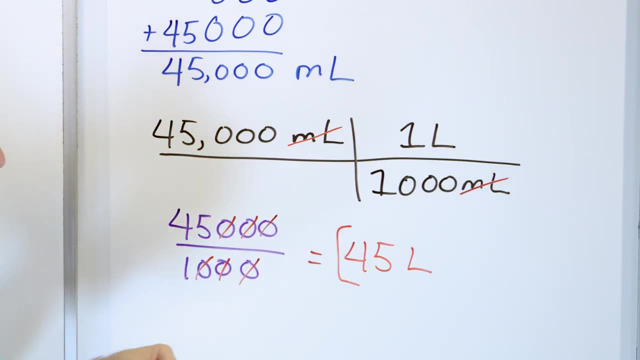 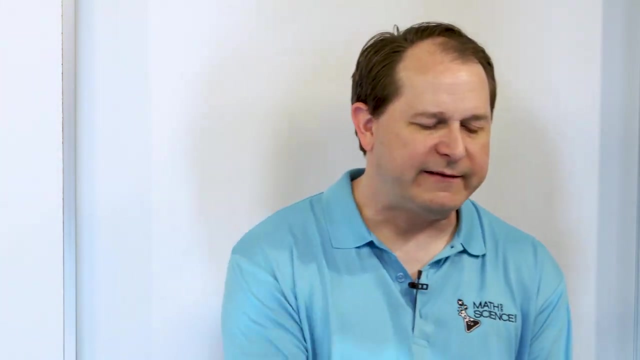 hard to know if you should multiply or divide to change units, But this way you will never guess. Arrange it so that the units cancel and we have liters left over, and then you'll be in good shape, no matter what. All right, only a couple more. They're not too bad. Let's take a look. It says there will be 84. 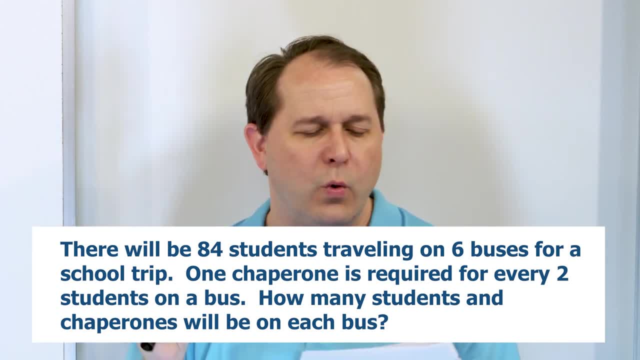 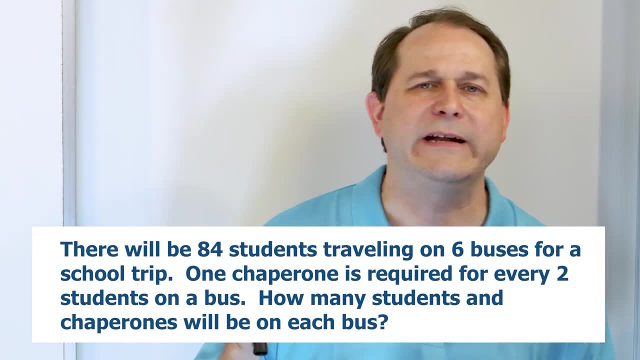 students traveling on six buses for a school trip. One chaperone is required for every two students on a bus. How many students and chaperones will be needed on each bus? So there's kind of two questions here: How many students on a bus, How many chaperones on each bus? So let's break it. 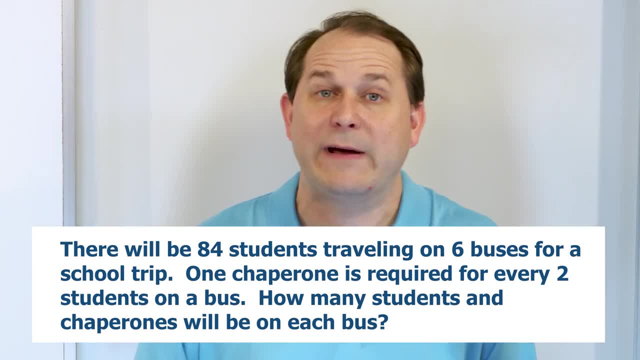 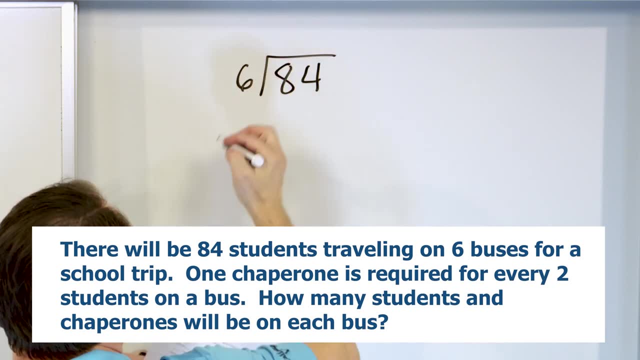 apart, 84 students on six buses. How many students on the bus We have to divide because we're dividing by six buses. So we'll take the 84, and we will divide it by six. All right, six can go into eight one time. 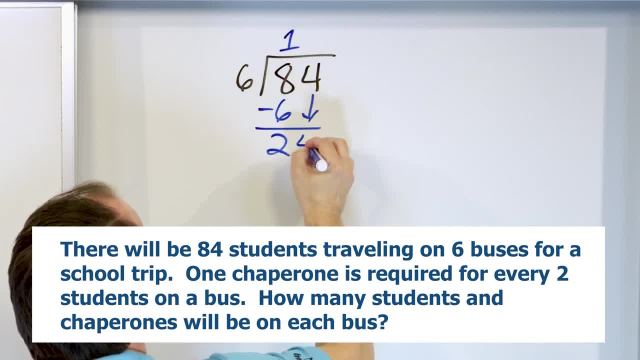 Multiply: get a six. Subtract: get a two. Drop this down of four: Six times one is 24.. Six times four is 24.. Subtract: get a zero. All right. so what have we figured out If we have 84 students? 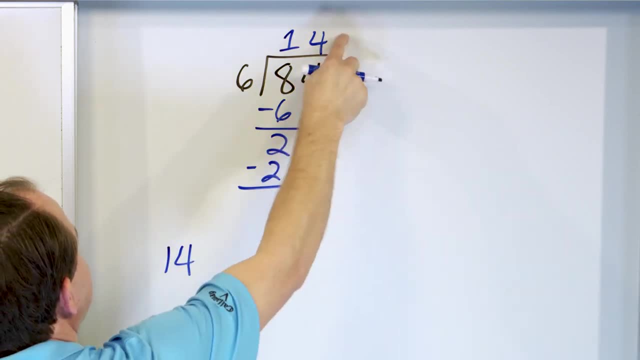 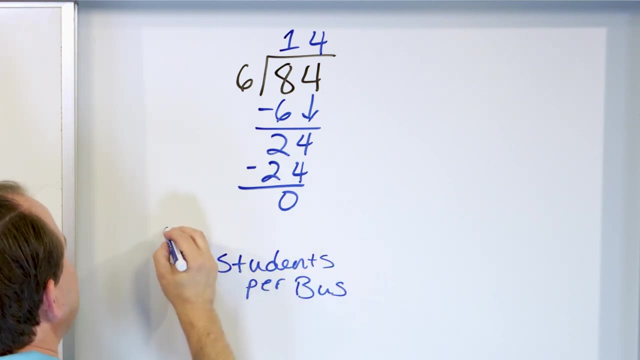 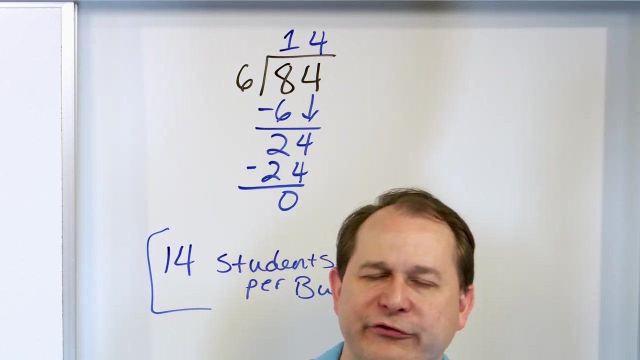 and six buses, then there's definitely going to be 14, which is the answer we got: students per Bus, All right. so that's one answer to one question. Now it says how many chaperones per bus. It tells us that one chaperone is needed for every two students on the bus. for every two. 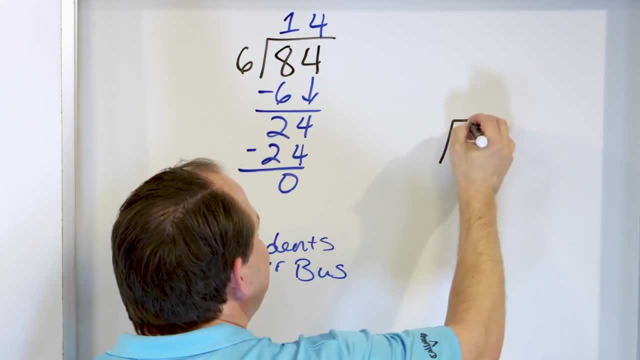 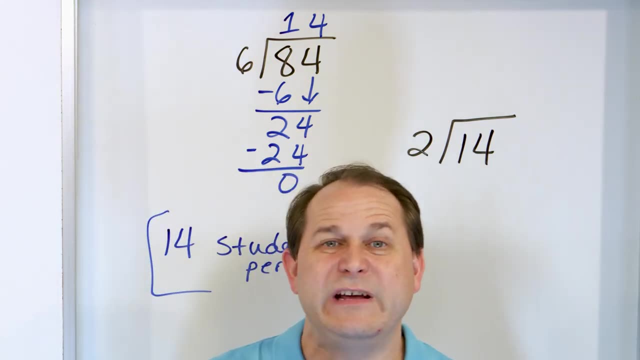 students. So if I know that I have 14 students, then I'm going to divide it by two to figure out how many chaperones I need. In other words, if I had 14 students and I needed one chaperone for. 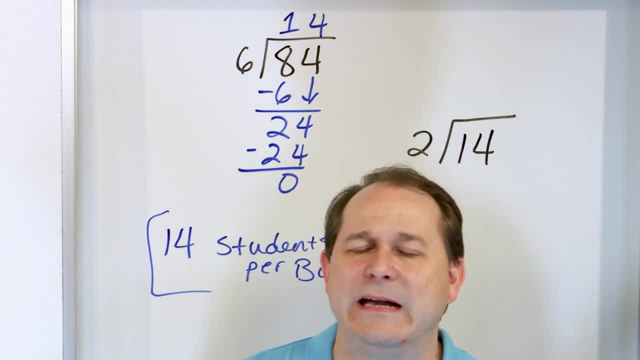 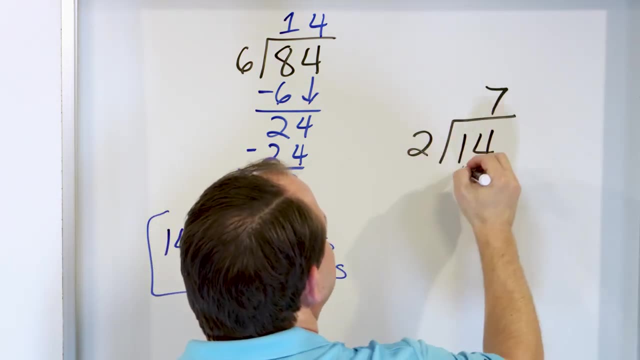 each student. I would need 14 chaperones, but I don't need that many. I only need one chaperone for every two students. So I'm going to divide that by two. Then, of course, two times seven is 14, and you can do the subtraction remainder of zero. So I'm 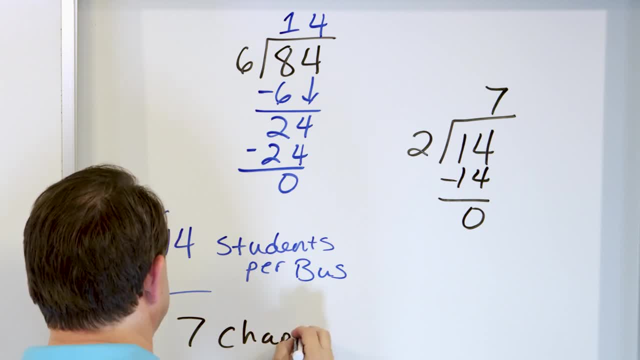 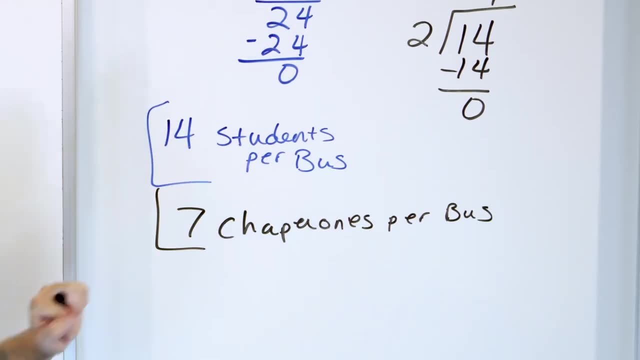 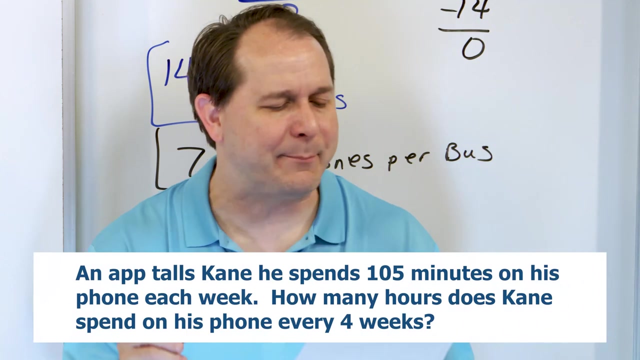 going to need seven chaperones per bus. So basically, on every bus you're going to have 14 students on the bus and you're going to have seven chaperones on the bus as well. All right, final problem: It says an app tells Kane that he spends 105 minutes on his phone every week. 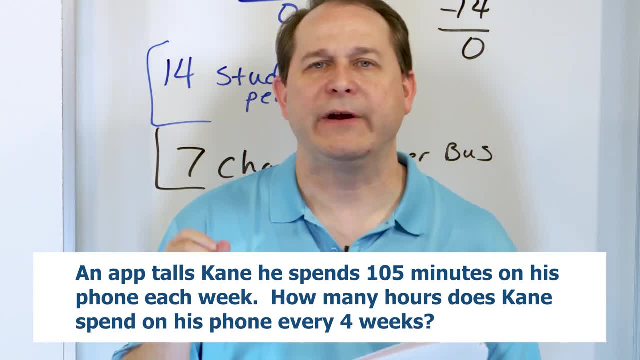 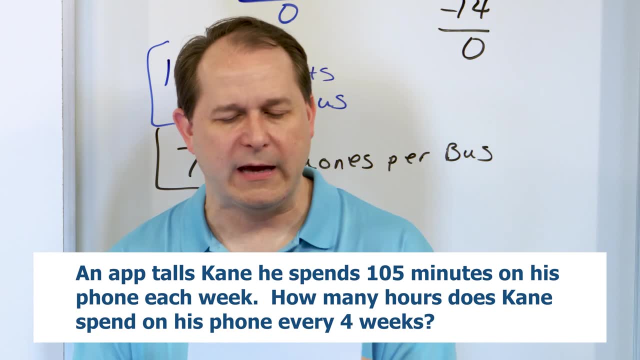 How many hours does Kane spend on his phone every four weeks, every four weeks? So it says 105 minutes on his phone every single week. How many does he spend every four weeks? So the first step is to take 105 minutes and we're going to multiply. 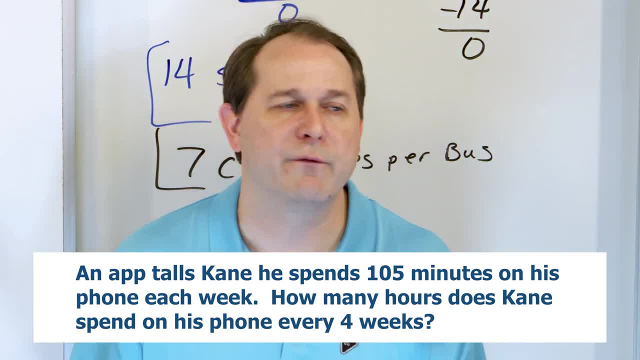 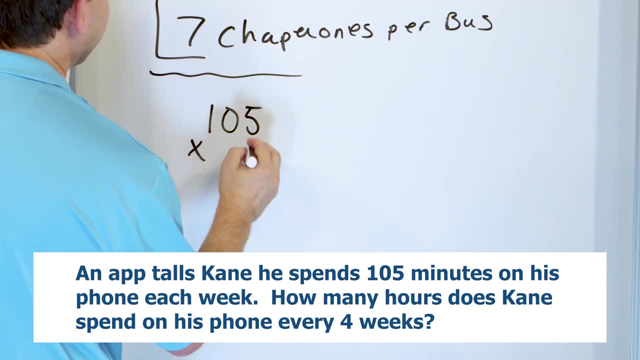 by four, because that's going to tell us how many minutes he's spending over the four weeks, right? Because it tells us in the problem statement that 105 minutes per week, and then how many over four weeks. we're going to multiply by four, All right. so five times four is 20, carry the two Four times. 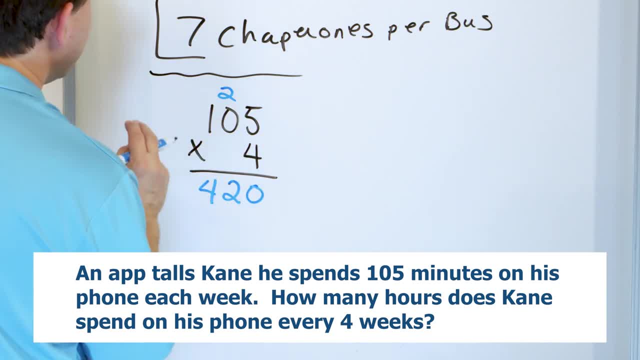 zero is 20,. carry the two, All right. so five times four is 20,. carry the two, All right. so five times four is zero, and then plus two is two, and then four times one is four, 420.. What do we measure? 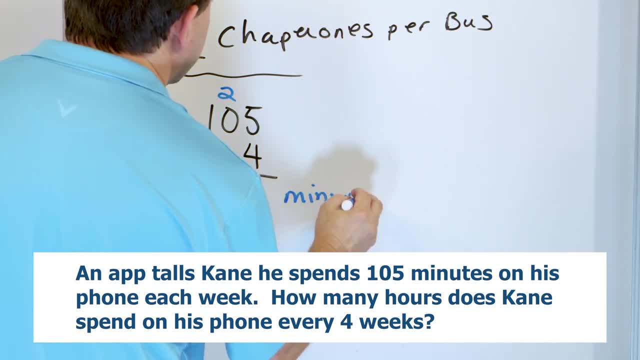 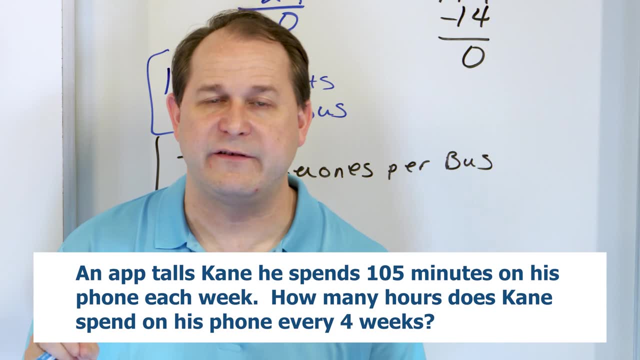 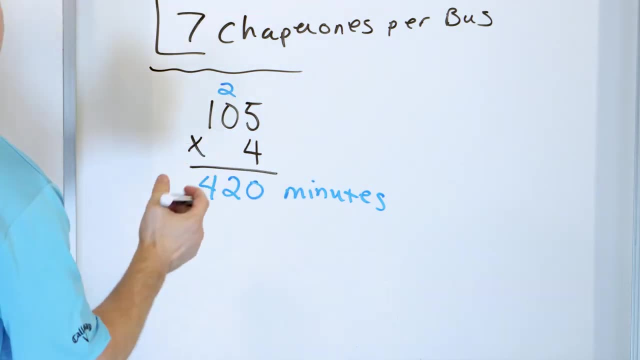 here: 420 minutes. 420 minutes over a four-week period. But the question is not how many minutes, how many hours does he spend over that period? So all we have to do is take this and convert it to hours. How do you do it? Maybe you're not sure, so set up a conversion. What you do is you say: